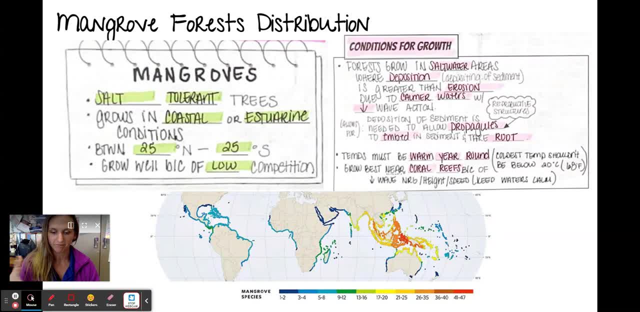 River Lagoon to the ocean, And then they'll get displaced again and we'll talk about how they can float in the water and how long that'll go for. So that's what we're going to be talking about. Temperatures need to be warm year round. Lowest temperature really shouldn't go below 68 degrees. 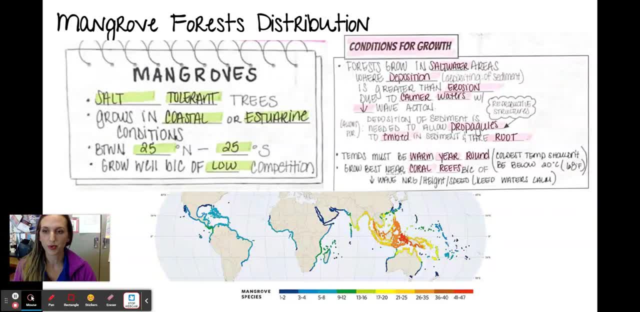 Fahrenheit, but we know that it gets a little bit colder here, but it's pretty warm around here all the time, and so is our water. They grow really good near coral reefs because coral reefs are going to be a barrier for wave action, And so when the wave action is low- and I have a picture- 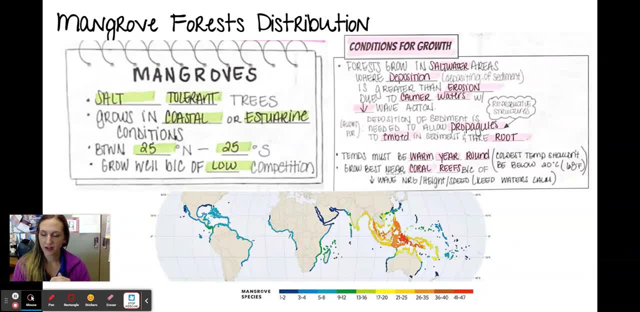 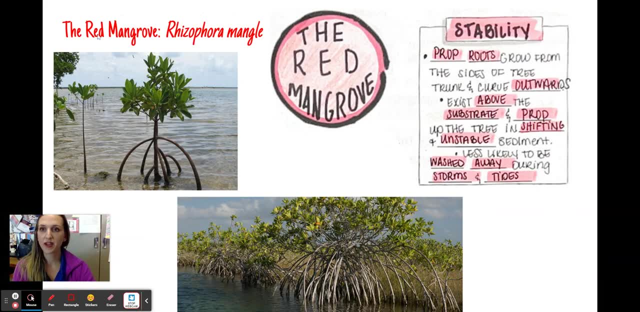 here to show that too. When the wave action is low, then you're going to have a lot more water. You're going to have a lot more sediment deposition. Okay, the mangrove species that we're going to focus on, and that is from your syllabus. 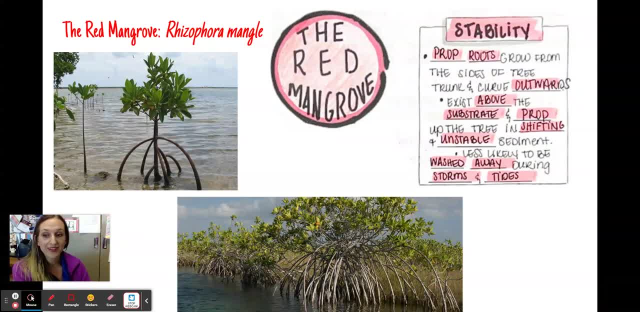 is Rhizophora mangle. And notice how it's written: It's in italics and the genus is capitalized. So some big features that we're going to have to reflect on are the prop roots, their root structure, prop roots: They grow from the side to the trunk, They curve outwards. 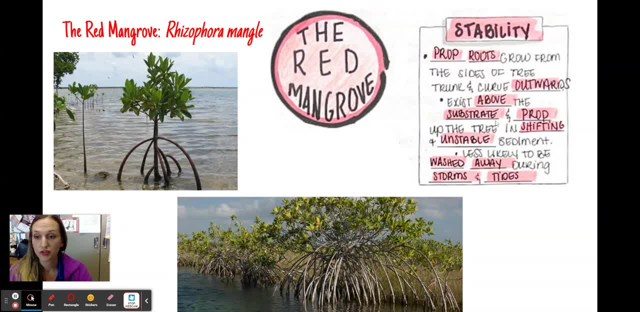 and then they exist above the substrate- And we'll talk about why in the next slide- And they prop up the tree and it helps them in a shifting or unstable substrate. So unstable substrates are going to be things that are very fine and that can experience some tidal. 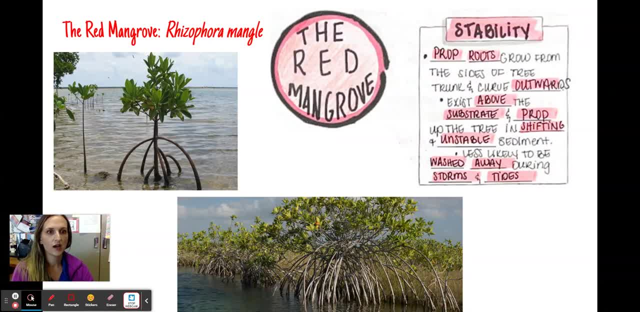 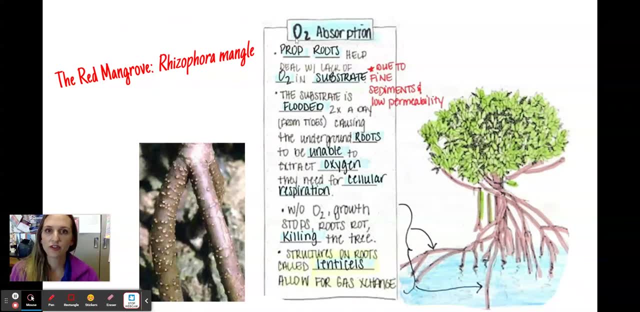 or some wave movement, some water movement, And so it's less likely to be washed away from storms or from tides. All right, oxygen absorption. So how do they absorb oxygen? The prop roots will help deal with the lack of oxygen in the substrate, because the substrate is very 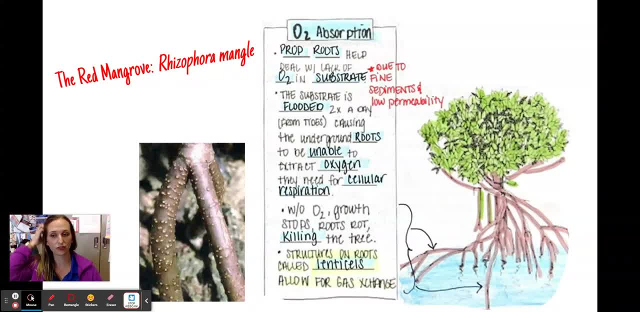 very fine sediment, fine sands, some coarse sands. There's also some mud there. If you've ever put your foot in our estuary it can get kind of thick. But for permeability of fine sediments it really traps gases in. It'll trap water from going through. It'll take a lot longer for water. 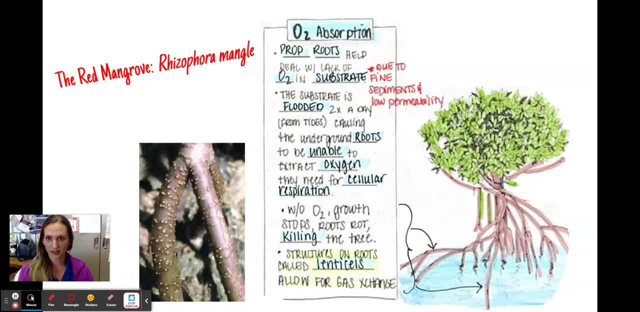 to go through, And so, if there is a lack of oxygen in the substrate, they got to find another way to get it, And so they Oops to the bottom. I'll just keep reading with it. The substrate gets flooded twice a day due to your tides. 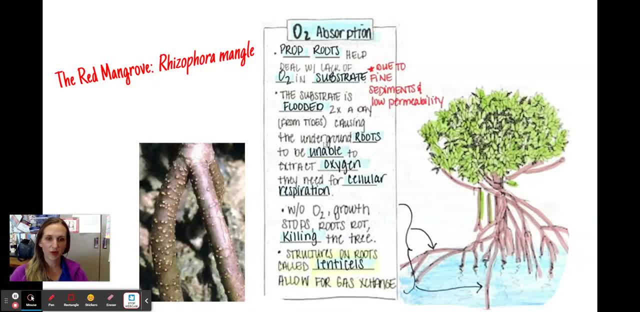 and twice a day will be semi-diurnal, And this will cause the underground roots to be able to extract oxygen from the water Again, because the sediment's so fine. Sometimes, when that happens, you can smell it. It might smell swampy And of course they need oxygen for cellular respiration. 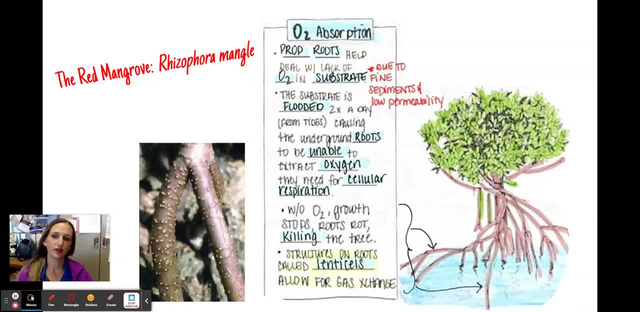 Without the oxygen, the growth will stop and the roots will rot. This will kill the tree. The structures on the roots are called lenticels- And you actually That's one of your vocab words- And this allows for gas exchange, And there's a picture right here, on the left side of this. 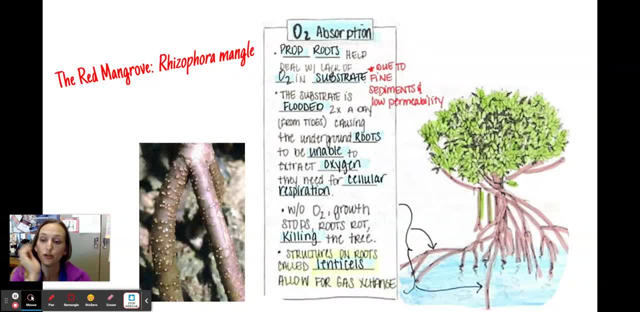 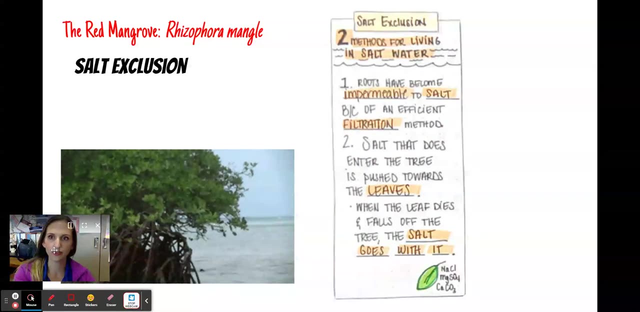 And those are the lenticels, And they actually can close up whenever they are inundated with water. So these exist on the roots, above the actual water line, so they can extract oxygen from the atmosphere. Okay, Salt seclusion. So living in a salty environment, how are they able to? 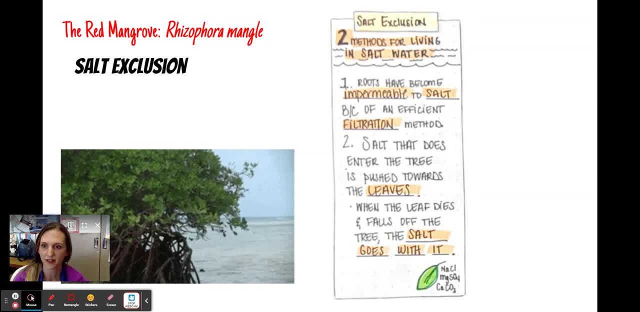 live and then not to lose water, because they're constantly around salt, so osmosis would force water to leave. They have two methods. One: their roots have become impermeable. So that's an adaptation that a lot of plants don't have. But their roots are impermeable to salt because they 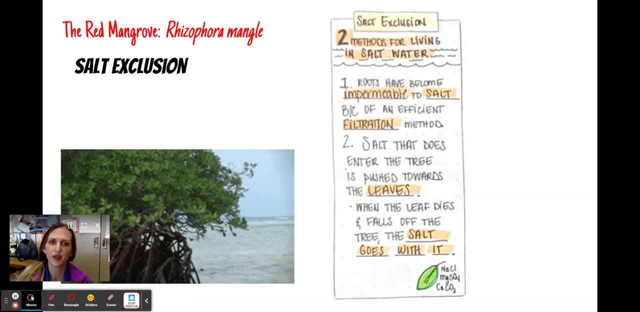 have a very efficient filtration method. Another one is salt that does enter the tree- And I believe it's like 97% of the salt- does not get through the roots. Salt that does enter it does get pushed towards the leaves And then when that leaf dies, it's going to fall off and the salt's going to go. 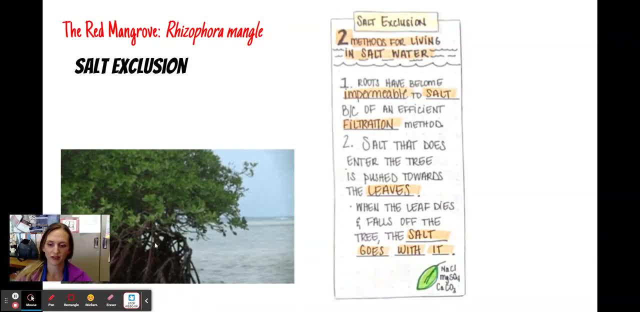 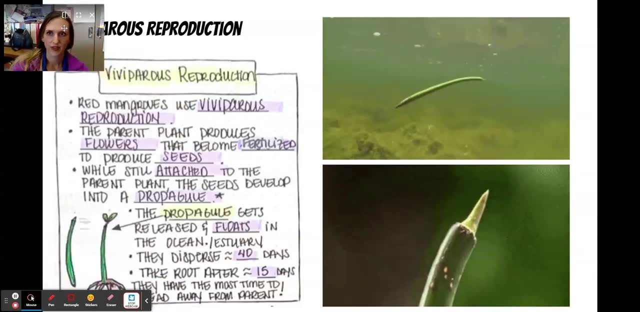 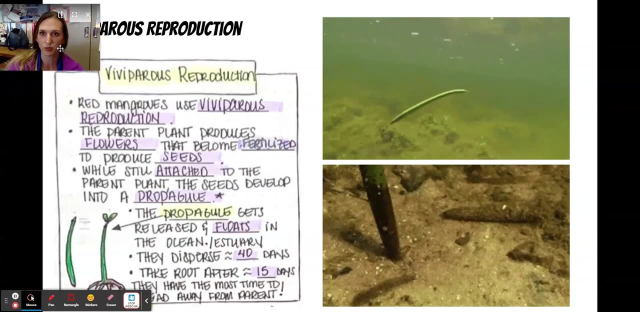 with it And then, just at the bottom, a reminder of the salts that are in your syllabus- sodium chloride, magnesium sulfate and calcium carbonate- And the way they reproduce: It's called viviparous reproduction. So use viviparous reproduction And the gifts you want to follow. 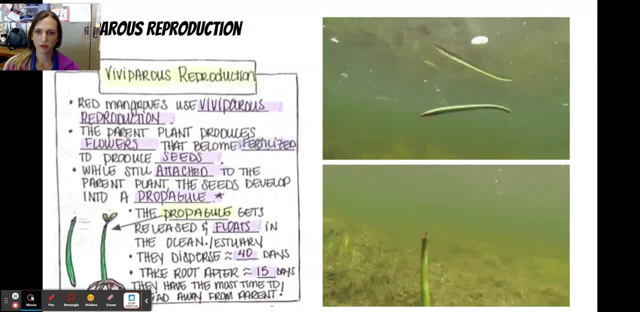 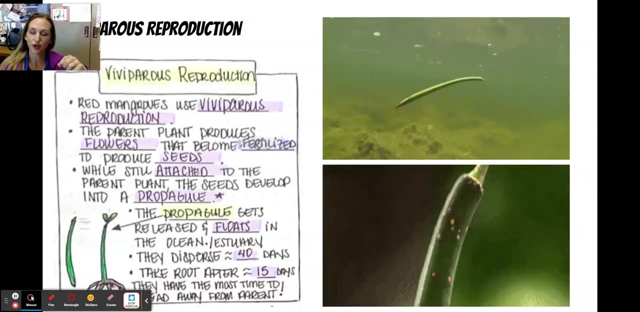 the one on the top and then the one on the bottom. So the parent plant will produce flowers. Those flowers will become fertilized And then they will produce seeds. And those seeds will grow into these elongated green propagules, little propagules, tiny little ones. So they have prop roots. On the roots are lenticels, And then they. 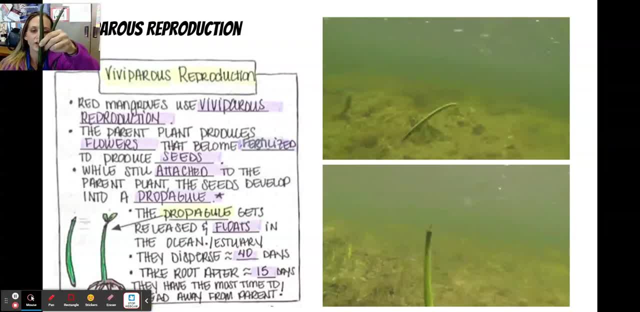 produce little seedlings called propagules, And they don't initially have the root structure on them. This is just because it's been sitting in water. Here's one with not a lot, But it's just because it's been sitting in water, And then they'll grow into these little propagules And 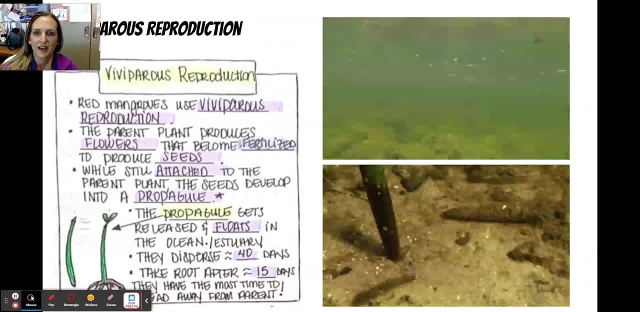 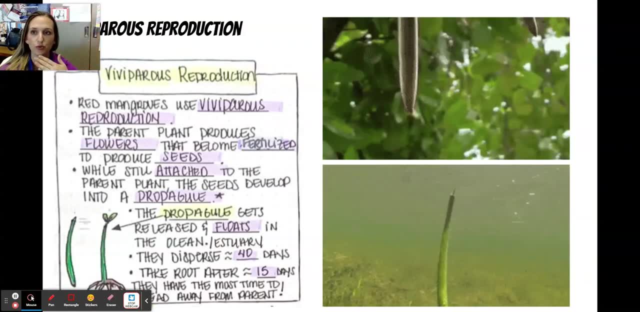 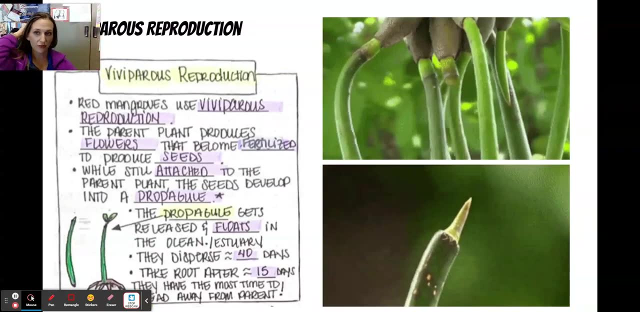 then they'll get into the water- Sweet little things, Okay, The propagule will get released And then it's going to be buoyant And it will float through the water, And then it will, after 40 days or so, they disperse themselves. They're going to move away from the parent plant, which is good. 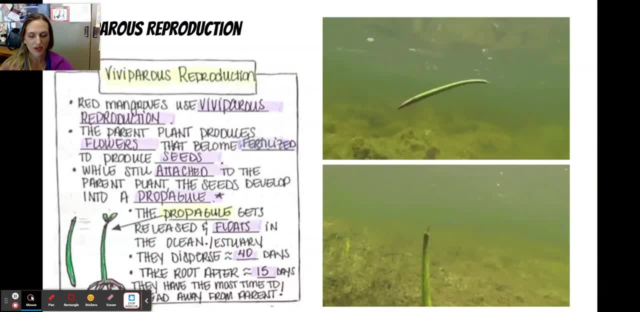 because you don't want the baby plant to be growing right by the parent plant, because then they will compete for space, compete for nutrients, et cetera. So you want them to be able to be dispersed away from the parent plant. So you want them to be able to be dispersed away from the parent plant. 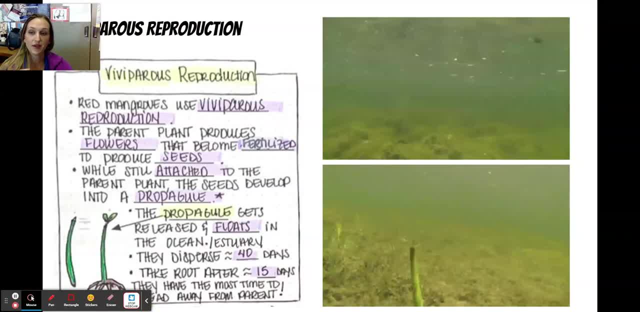 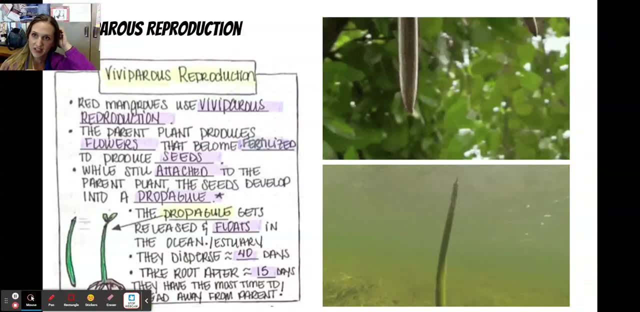 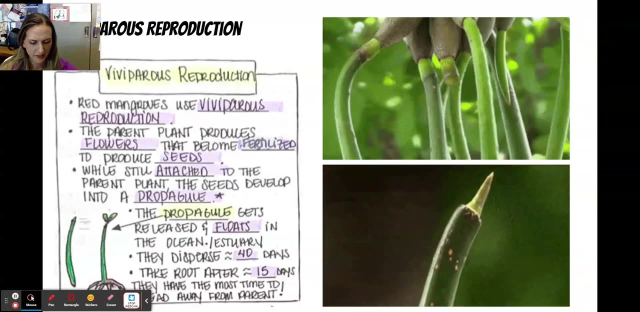 And then once they find soft sediment, if they do, but once they do find soft sediment they'll embed in it And then they can take root after about 15 days. And this is referred to as obligate dispersal, just in case that's referenced anywhere. It's not a vocab word, but in case it's. 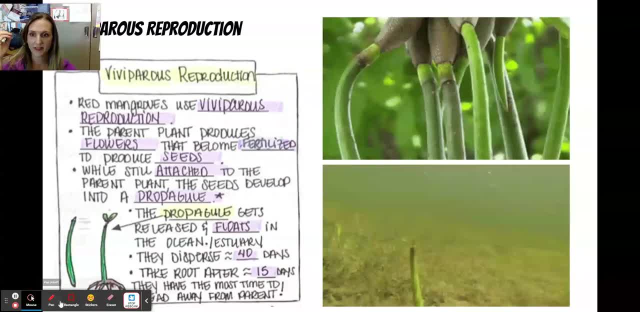 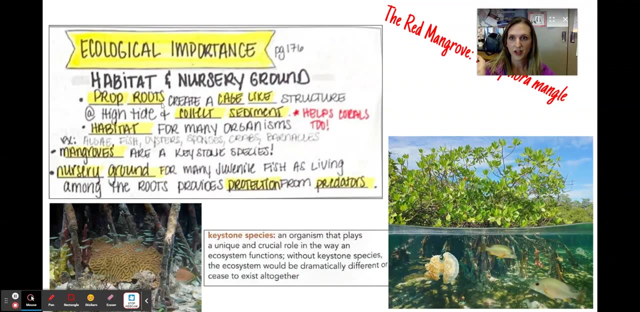 referenced Obligate dispersal. They also can float around the ocean for like an entire year and still be able to take root. Okay, the ecological importance. And again, we're still talking about the red mangrove, So the proper roots that create like a cage-like structure at high tide. 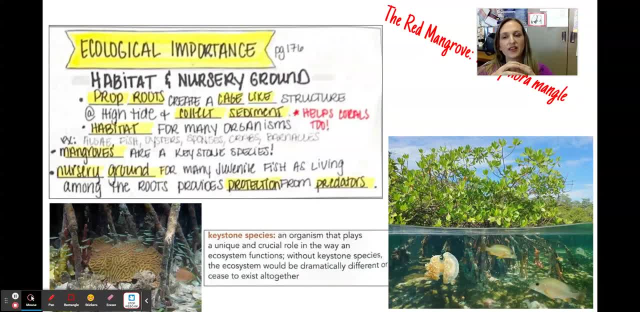 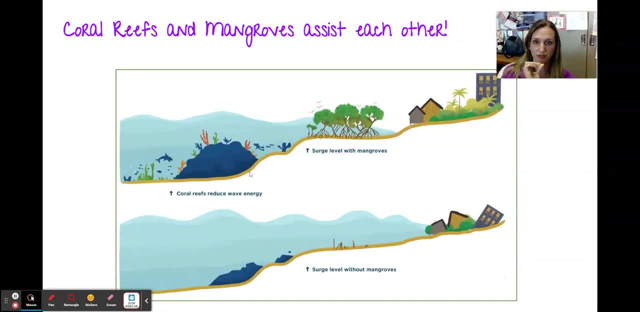 this will collect sediment. This is a habitat for a lot of organisms And they work so well with corals. I'm just going to go to the next slide really quick. So, like during a storm surge, the picture on the top is coral reefs will reduce. 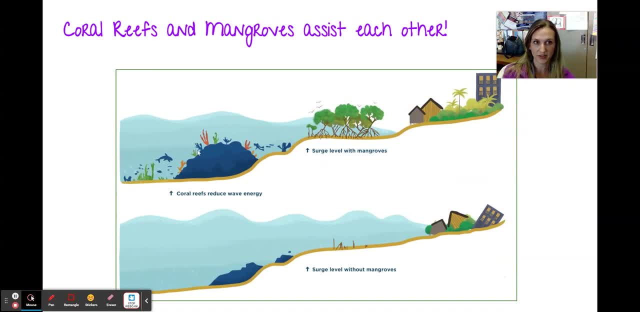 Wave energy. So if there's corals there, the waves are going to already kind of be slowed down from that. And then you have mangroves in front of it, So the corals are going to slow down wave energy so that it's not going to erode away the proper roots. And then, with the mangroves there, 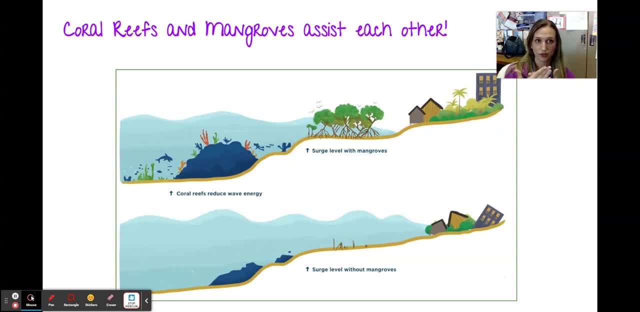 again. they have like a cage-like root structure that's going to further slow down the water And it's also going to trap sediments and they can start depositing and build up land Without mangroves. you might have your corals there And it really doesn't look biodiverse at all. Looks like there's. 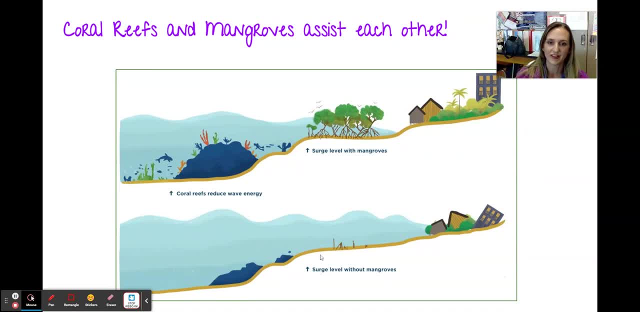 some damage. But with the corals without mangroves- not there- obviously you're going to have some destruction, because there's really nothing to slow down that wave energy at all. In addition, corals need sunlight And because the mangrove roots act like a cage, 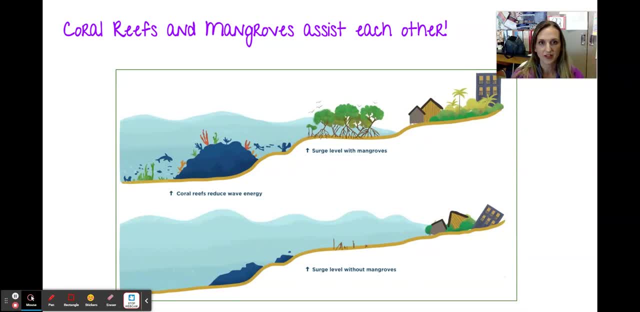 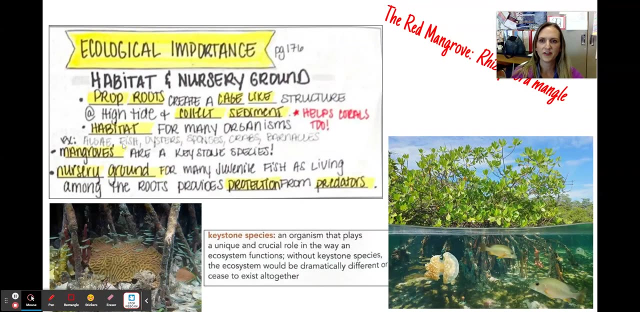 they are able to slow down water and trap sediment, So that sediment does not get dislodged within the coral polyp itself and then block sunlight. Okay, back to you. So habitat for many organisms And, like fish, oysters, sea sponges, there's some sharks there. 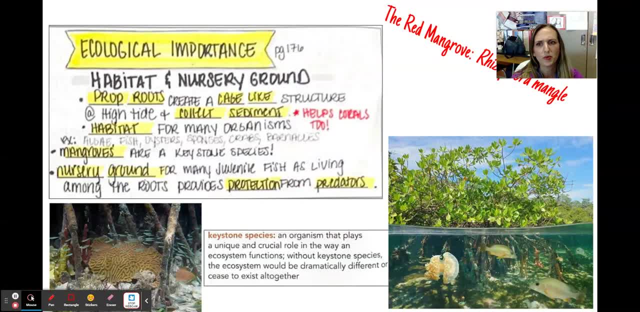 dolphins. We have a lot of dolphins in our river, Crabs, barnacles. They're a keystone species. because of that, You got your definition down here. All producers are keystone species because if you take them out of their habitat there's going to be a very negative effect. They're a 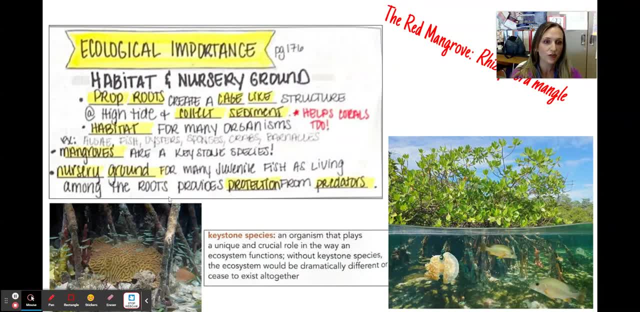 nursery ground for many juvenile fish, And so they're going to be a very negative effect. They will hide among the roots, which is good for them, because there's going to be oxygen coming from the plant doing photosynthesis that will allow them to do cellular respiration. 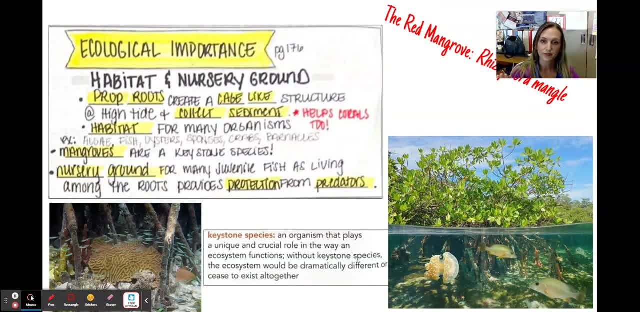 It's also going to be a source of organic material, because they're producers And they can hide among the roots and it protects them from larger predators. So we would refer to mangroves as a nursery ground for more juvenile fish And then, depending on the species, as the 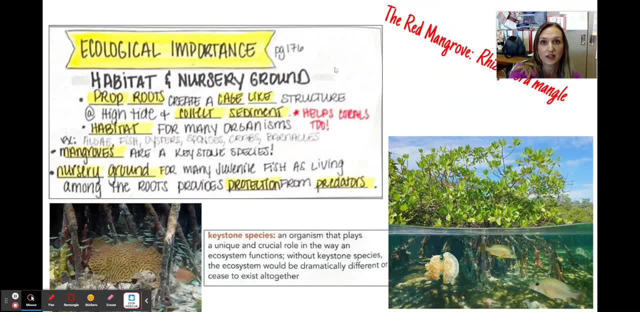 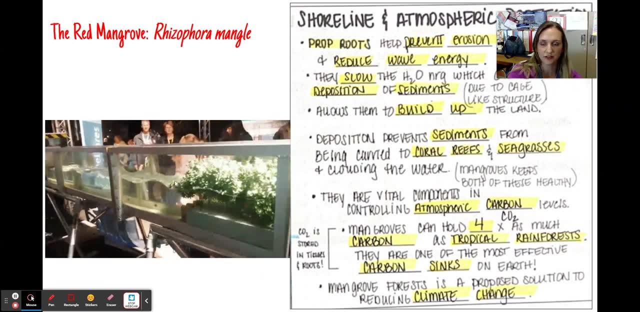 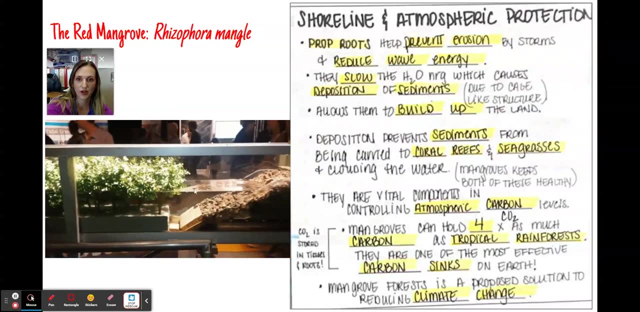 fish get older, they can move out to the big leagues, They can move out to the ocean. Okay, I always loved this GIF- Just prefacing that, Loved it so much. Oh, cool, I can make some more Great. Okay, Just so you can see on the GIF, here's some waves being propagated And then 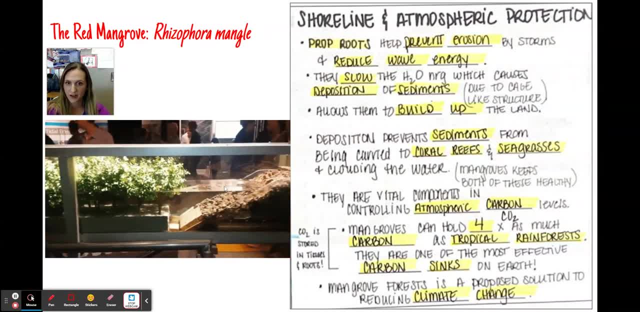 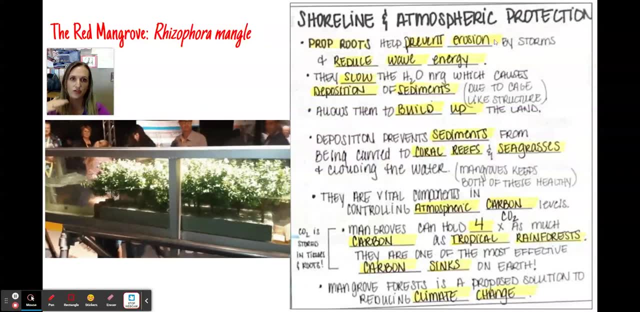 the simulated mangrove forest And notice the lack of water movement on the shore. Just a fabulous GIF, But propagates will prevent erosion by storms. They're going to reduce wave energy And then they're going to be able to move around the shore, And then they're going to be able. 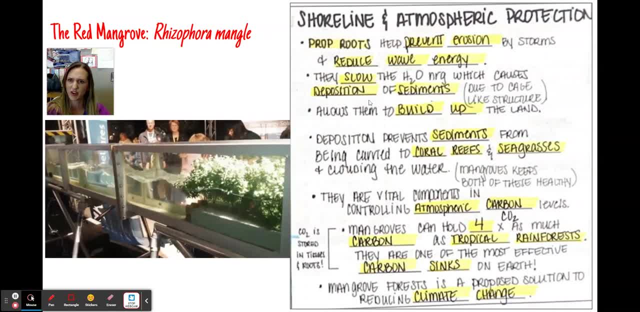 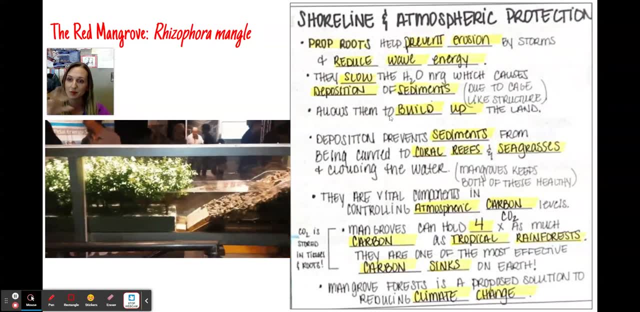 to move around the shore And then they're going to be able to move around the shore. They slow the water energy, which is going to allow for deposition of sediments, And we've covered a lot of that back in February. This will allow them to build up the land, like I said, because sediments 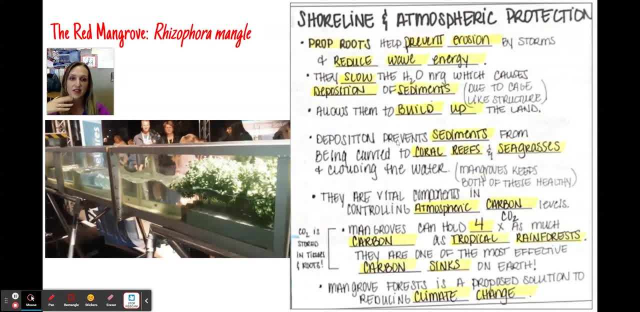 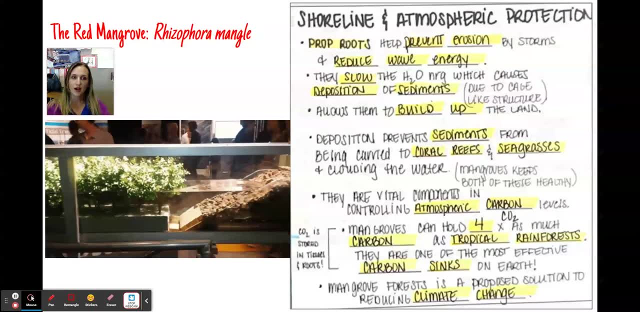 are going to slow down, get trapped and then deposit. The deposition is going to prevent sediment from being carried to coral reefs, like I said, where it can clog the coral polyps and prevent sunlight penetration. Additionally, same thing with seagrasses: The sediment can start. 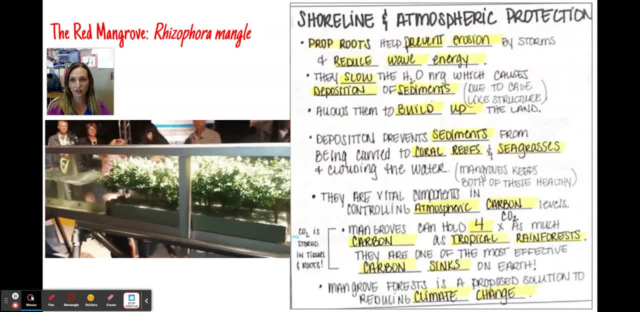 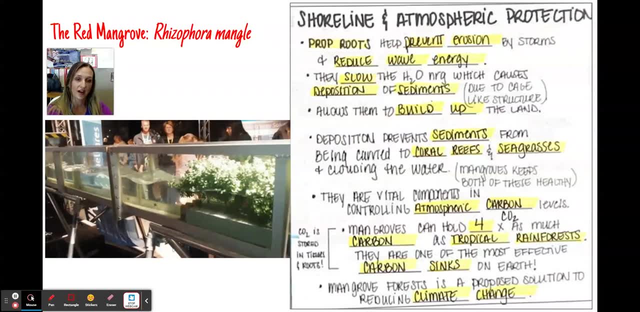 landing on the blades of seagrasses And then it's going to smash them, but also prevent sunlight. You don't want the turbidity in the water. They're vital components in controlling atmospheric carbon dioxide levels. They can store about four times as much carbon as tropical rainforests. 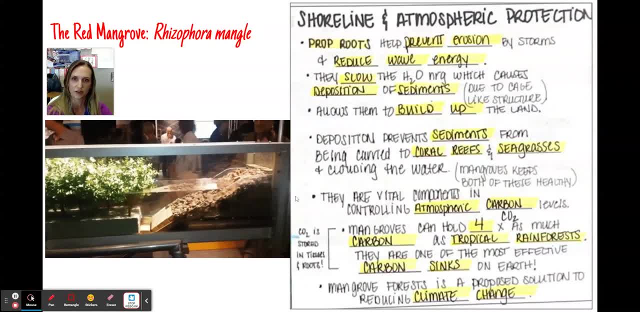 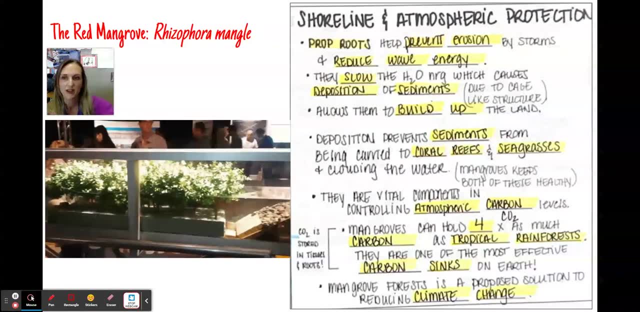 And they're one of the most effective carbon sinks on Earth. A carbon sink is a place that carbon will get stored. Mangrove forest is a proposed solution for reducing climate change because they can store so much carbon And not just in their tissues like within their 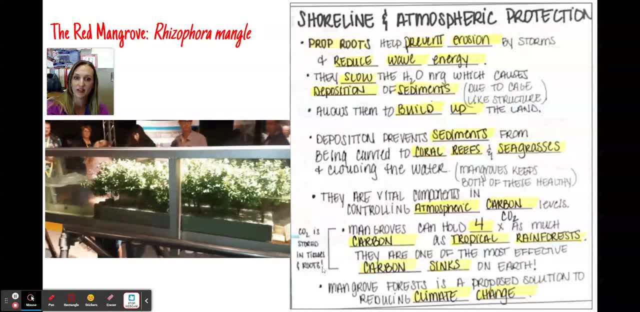 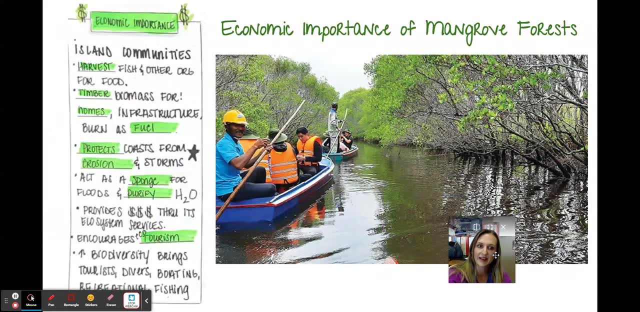 leaf tissues and the vascular tissues, but within the roots themselves. The roots can store even more The economic importance, so how they can bring money. So island communities will harvest fish and other organisms for food. Same with us. We're on a small scale, though We don't have any kind. 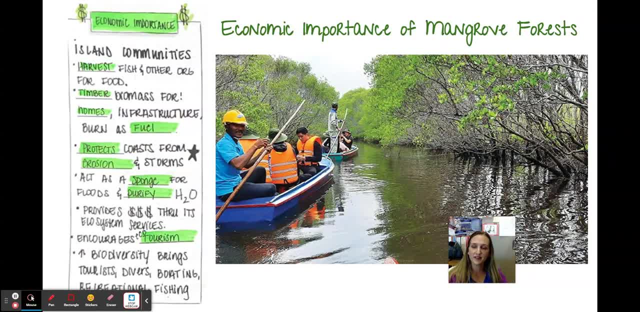 of like industrial fisheries, Timber used for biomass, or timber biomass used for building homes, Infrastructure. it's also burned as fuel And again, this protects the coast from from erosion and storms, And we have hundreds of millions of dollars in storm damage just. 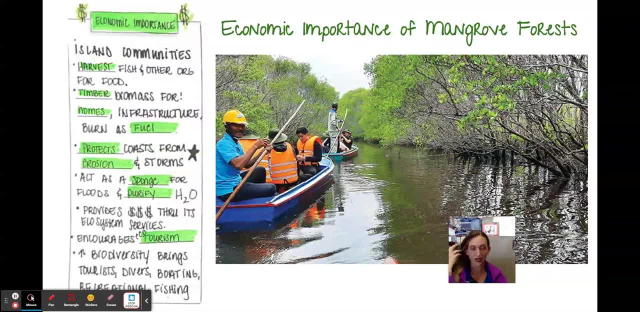 from those two Hurricane Ian and Hurricane Nicole that we had in Florida. So adding mangroves is just an extra protection to slow down wave energy and help with storm surge. This provides money through ecosystem services. So shoreline protection, climate control. 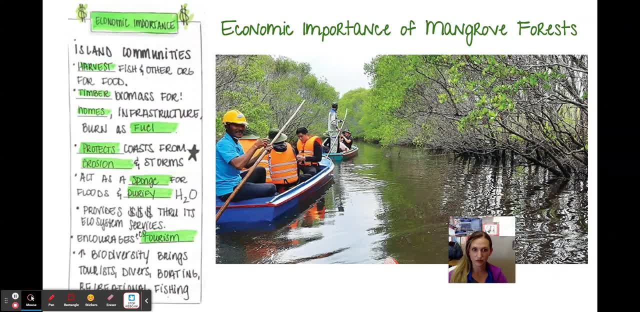 medicine, like proposed medicines, and we just discussed the biodiversity, you guys actually biodiversity assignment and food sources. um, this also could encourages ecotourism and even here, so when people go and see like the bioluminescence, when that happens in like september, october. 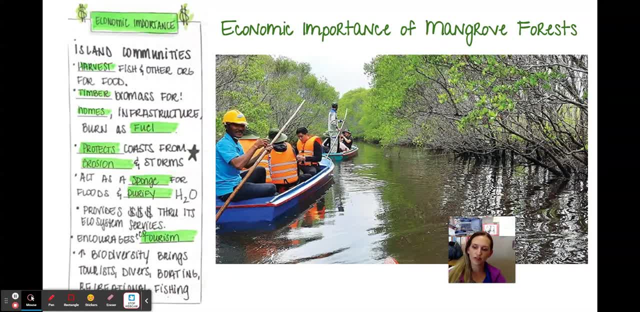 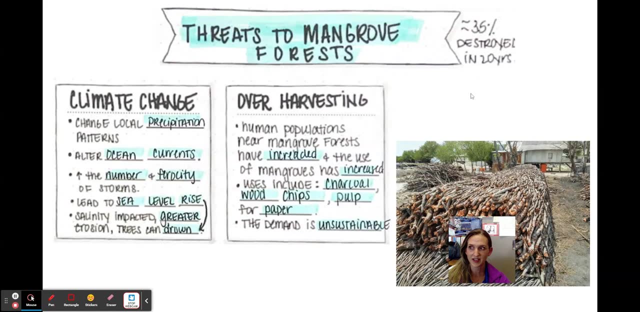 um, you know our local communities make money off people going to do that and we really can only have that because of the ecosystem that's here um. it brings tourists, divers boating and recreational fishing threats to mangrove forest. so since um 19 between 1980 and 2000, um about 35 percent of 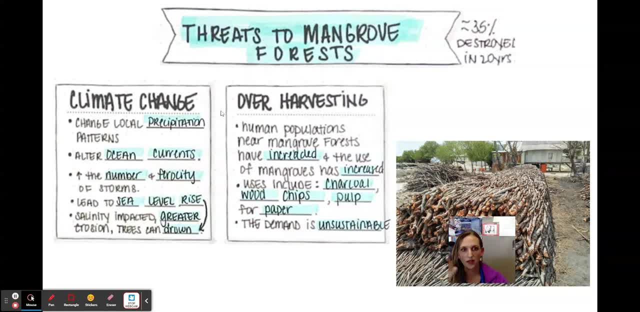 mangroves were destroyed and we'll discuss why in here. but threats to mangrove forest, climate change. so climate change can cause change in local precipitation patterns. um can alter ocean currents. remember currents is a continuous movement of water in a direction. um it will increase the amount in the ferocity of the mangrove forest and increase the amount of. 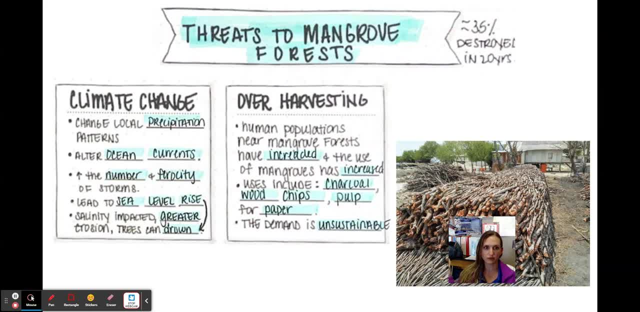 water. in the ferocity and the strength of storms which we've also seen all over um, it can lead to sea level rise and then back to where. if they stay inundated and they can't get oxygen, and if those lenticels are um are covered, then they're gonna be able to extract oxygen from the atmosphere because 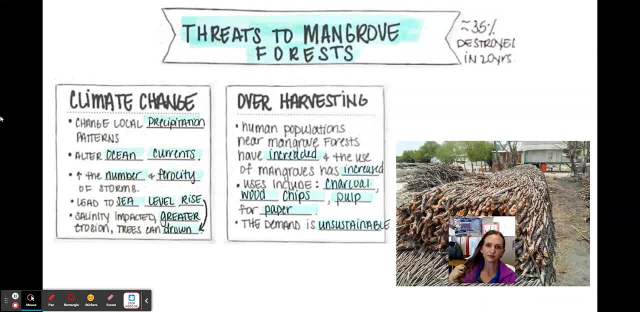 sea level rise, um, they're gonna end up drowning. uh, over harvesting is another one, so cutting them down. human populations near those forests have grown, so so has the harvesting of mangroves. um, the uses for them are for charcoal, um for wood chips, for pulp to make paper. the demand is. 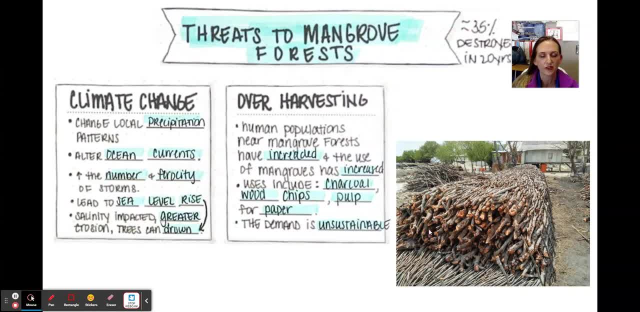 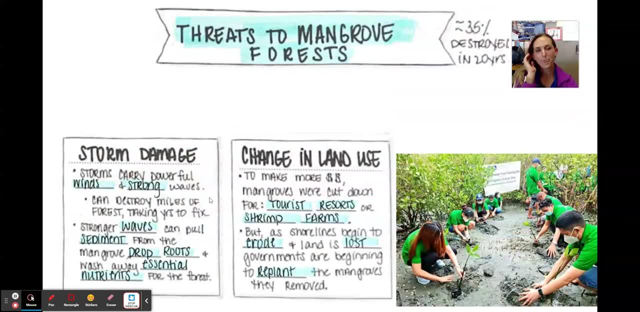 unsustainable, and this actually was a picture that was mangrove trees being cut down for use of charcoal or to produce charcoal. last slide, um, from storm damage. so storms carry really powerful winds and strong waves and this can destroy miles of forest. stronger waves are going to erode and pull. 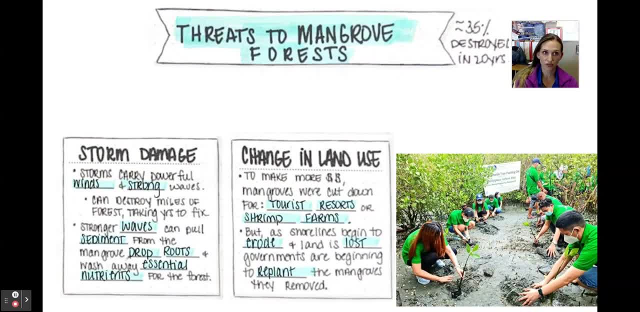 away from the mangrove forests, um. so the mangrove trees are going to erode and pull away from the crop roots, um, which can obviously wash away the entire plant and it will extract nutrients that would be essential for the entire mangrove forest. lastly, another threat is going to be changes in 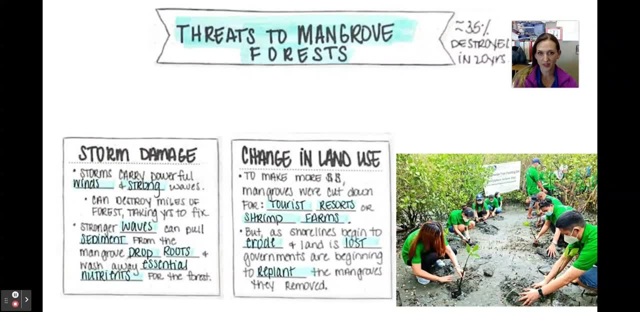 land use so to make more money. initially mangroves were cut down. they were unsightly and they smelled bad because they live in fine sediments that trap gases. um, so places started to cut them down and it would cut them down for building tourism resorts and shrimp farms and which i'm sure those 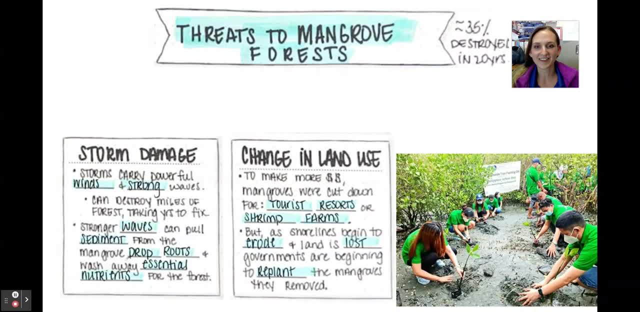 smell even better. um, but then they noticed that their shoreline was starting to erode. um, land is being lost, and then, through further research, we know that mangroves are a massive solution to that. so governments are beginning to replant mangroves that they removed.